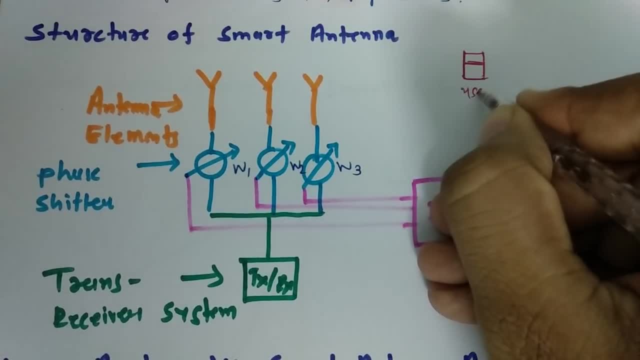 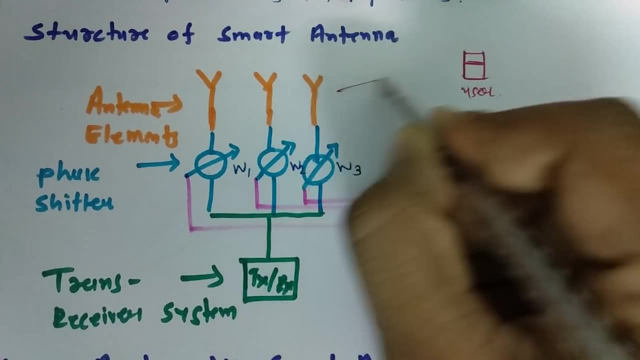 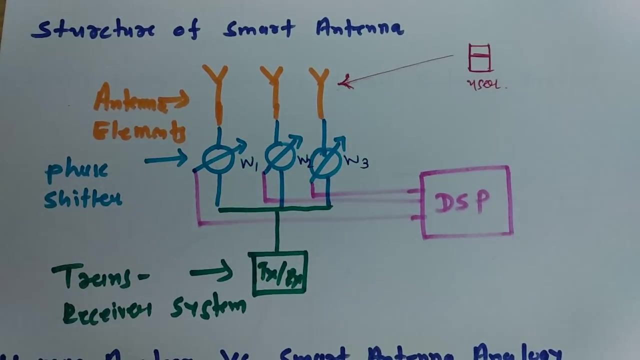 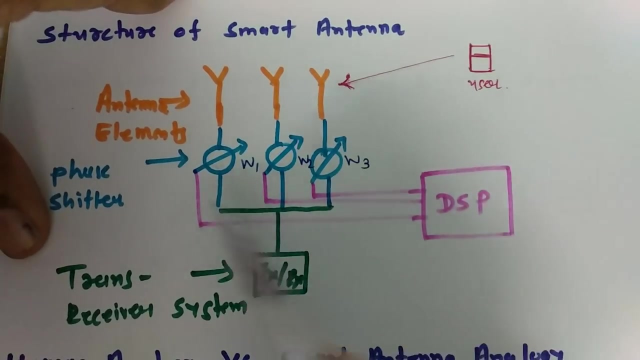 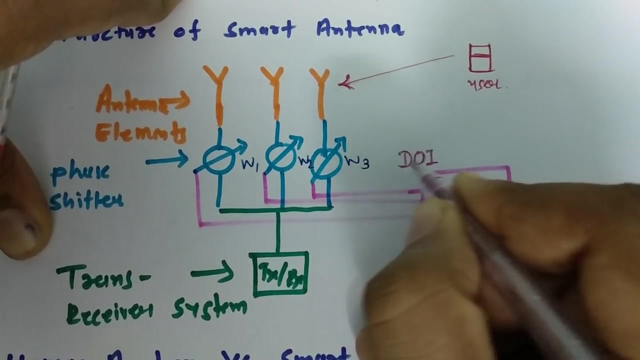 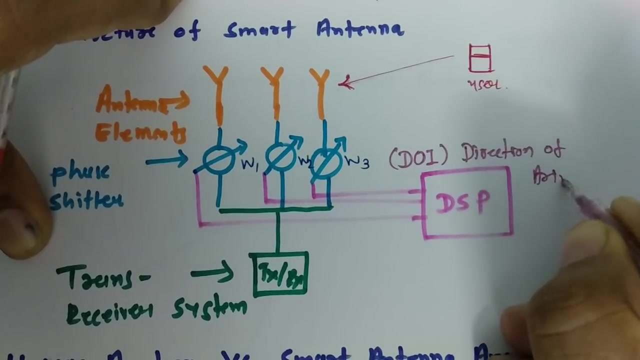 is, i am placing one user over here. now what happens is, when this user sends signal to our system, then this signal that is coming from this direction and here, based on signal reception, this smart antenna dsp processor will justify direction of arrival. so direction of arrival, of arrival. 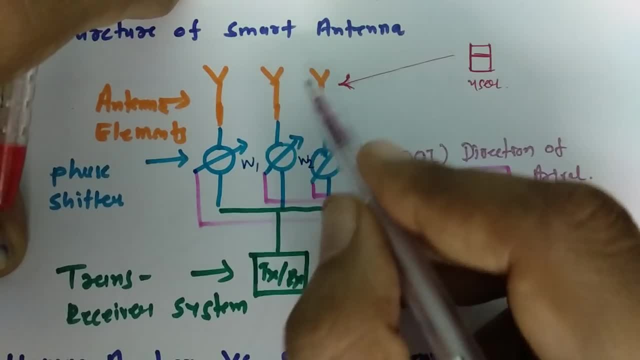 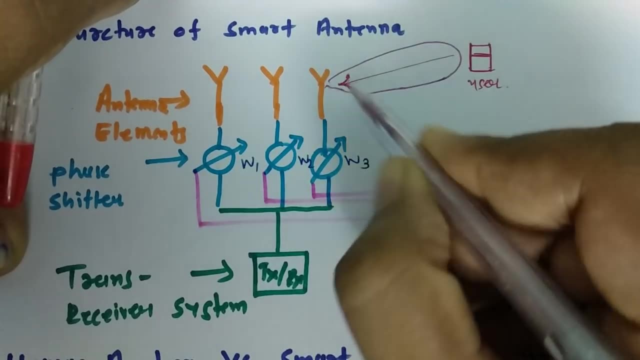 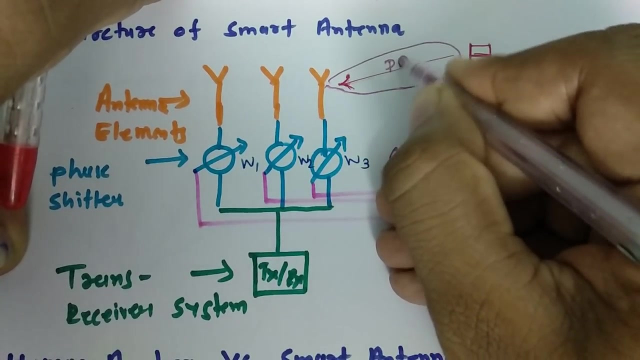 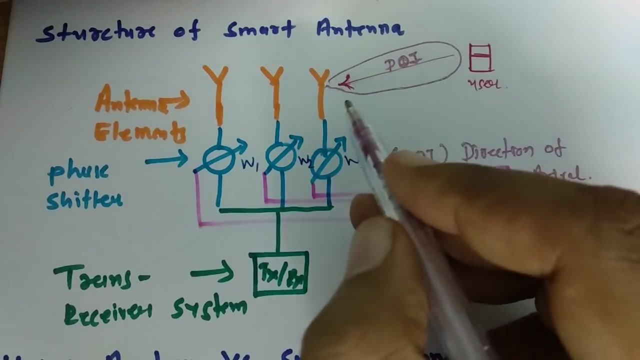 of arrival, elements that will be sending signal in this direction only. So main lobe that will be there in this direction only and that is based on direction of arrival. So, ultimately, what happens in this smart antenna structure? it radiates in intended direction, only It radiates in intended. 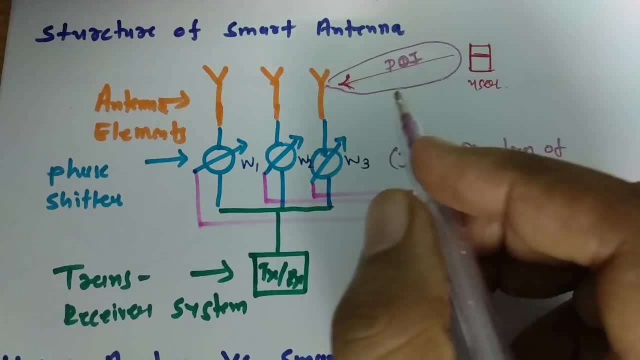 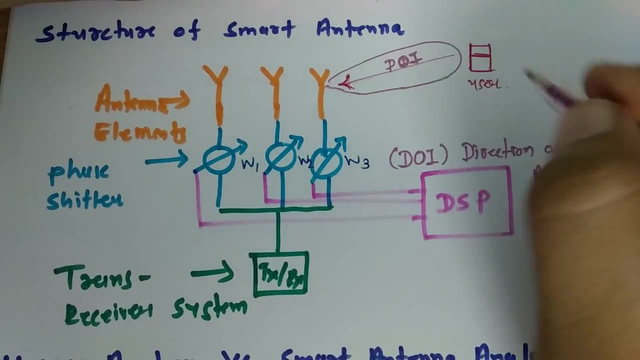 direction only and here it will be having minimum effect of interference. So these are the basic feature which is there with smart antenna, Based on the user direction it radiates. So first this system will identify direction of arrival and once the system justifies what is the 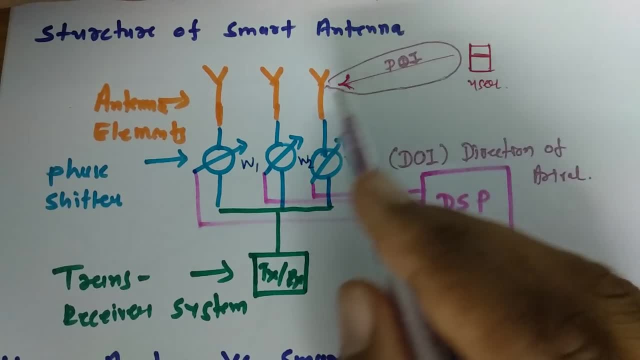 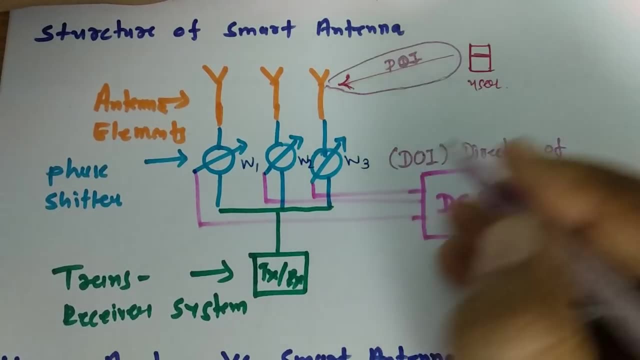 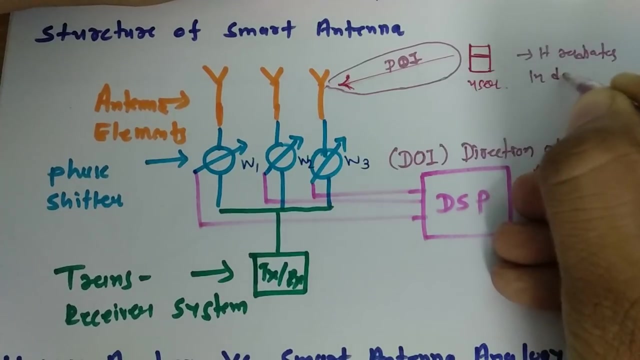 direction of arrival. it will be sending signal in that direction only. So it justifies The direction, which is what desired direction? So it radiates in desired direction, only It radiates in desired direction. So it radiates in desired direction, and because of it radiates in desired direction, there will be minimum interference. 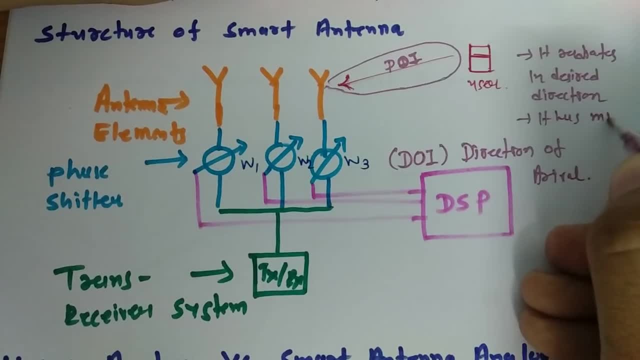 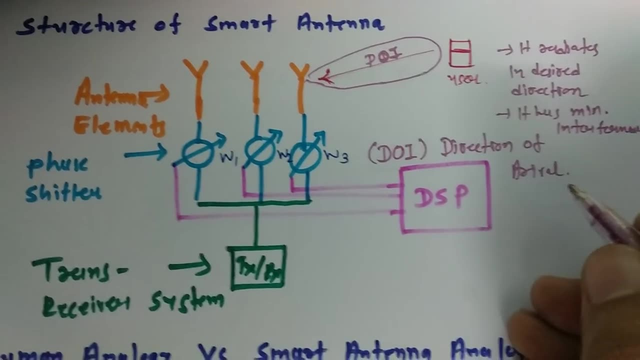 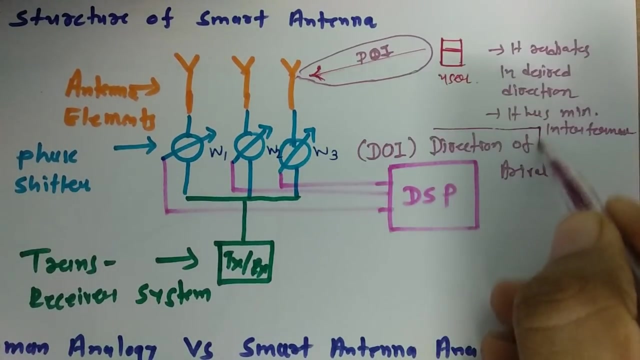 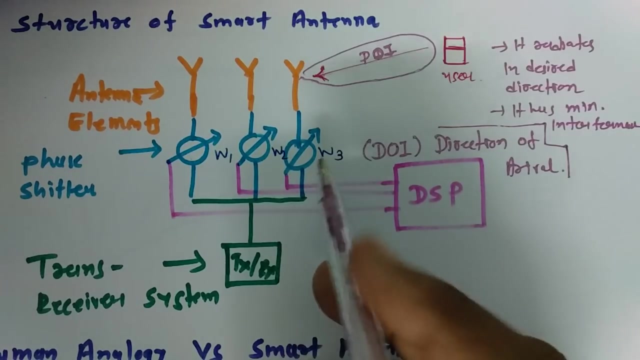 So it has minimum interference. So it has minimum interference and it radiates in desired direction. and it radiates in desired direction based on direction of arrival. So that is how this smart antenna structure functions. Let us again have a quick review. Smart antenna structure that consists phase direction. 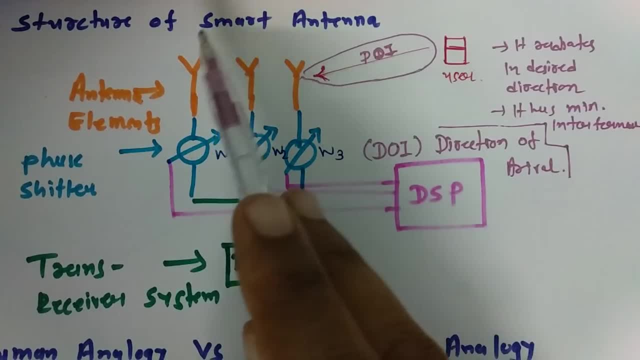 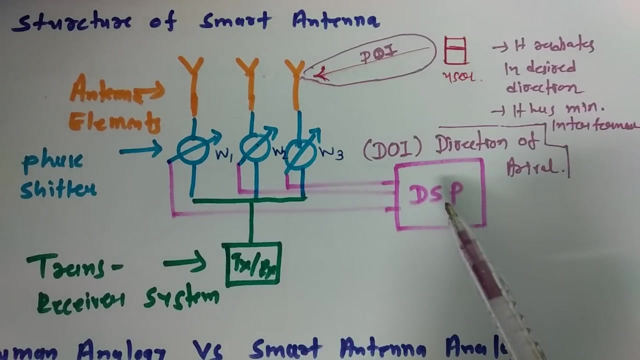 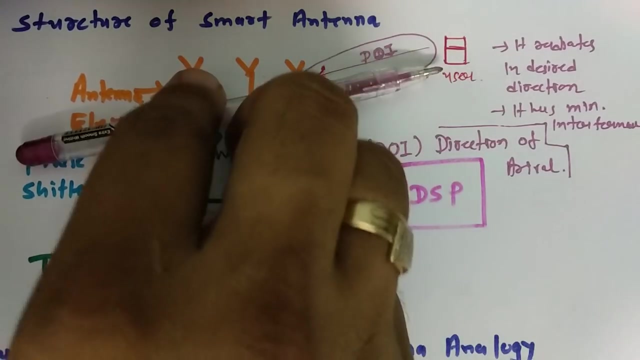 This is what a diagram of phased array where there are multiple antenna elements. Each antenna element is connected with phase shifter and then it is connected with trans receiver system, But this magnitude of phase shifter that has been justified by DSP processor. So, based on DSP processor magnitude given to this phase shifter, this beam is getting steered. 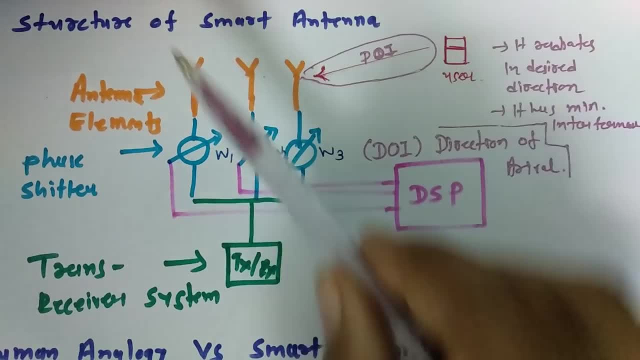 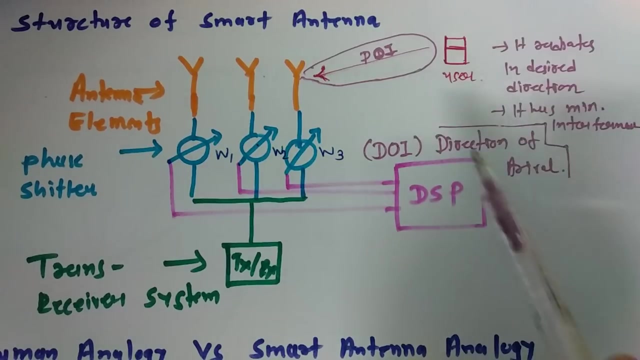 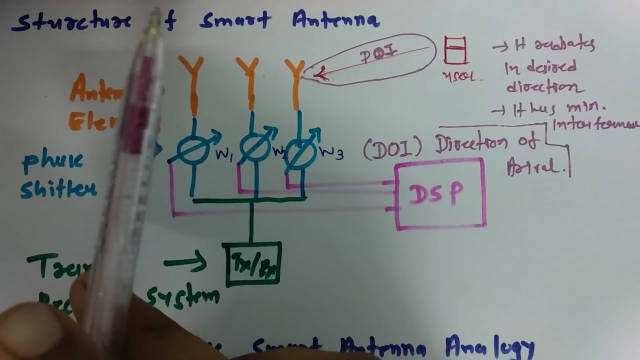 For example, if I say I have a user in this direction, then by changing the value Of magnitude of this phase shifter it will be steering beam in some other direction. So first, this smart antenna justifies what is the direction of arrival and, based on direction of arrival, it justifies angle of beam. and based on it justifies angle of beam, it radiates in intended direction. 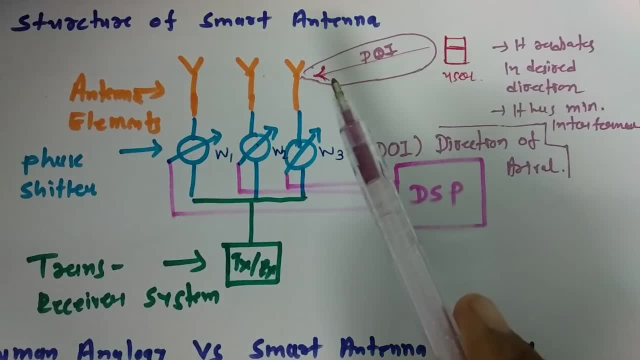 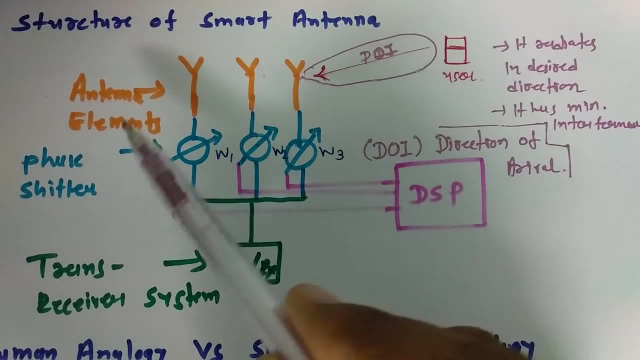 So it radiates in desired direction and because of it radiates in desired direction, it has minimum interference. There are few more features which is there with this smart antenna. One is it has minimum interference. Second is it has higher gain in desired direction. 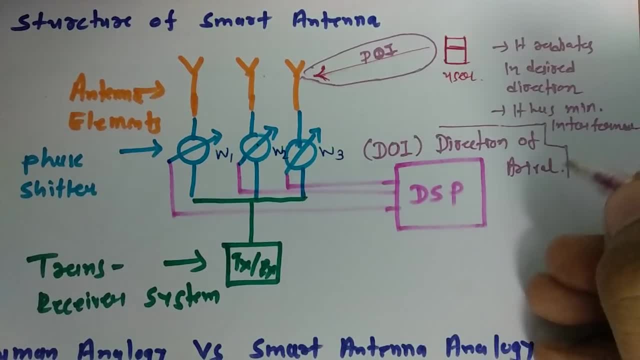 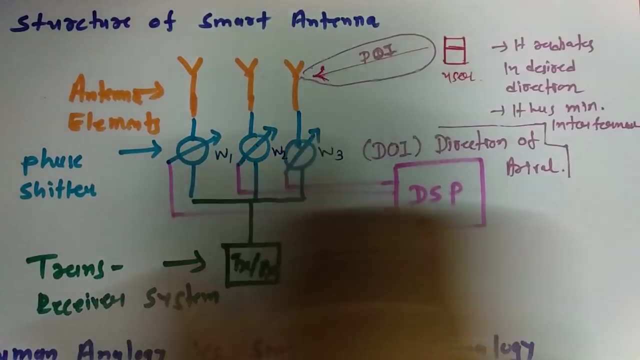 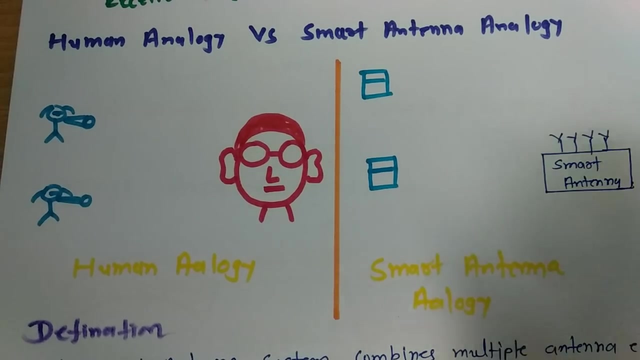 So it has, because of it radiates in desired direction, it has higher gain in desired direction. So this is how this smart antenna technology functions about. Now let us have human analogy with smart antenna analogy. Now here one can clearly see that is one human and there are multiple speaker. 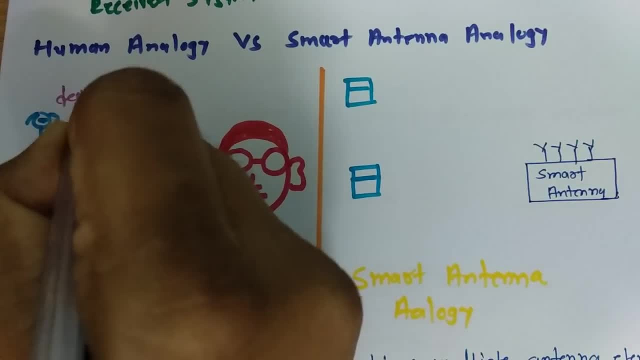 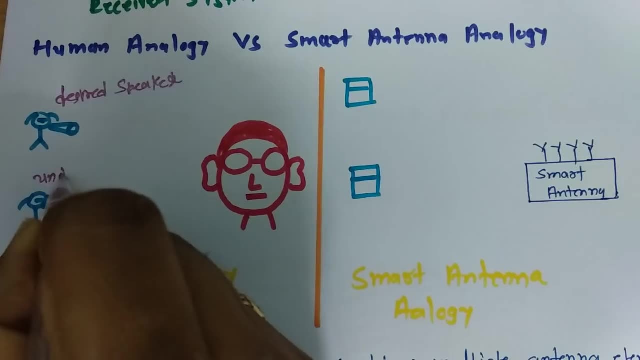 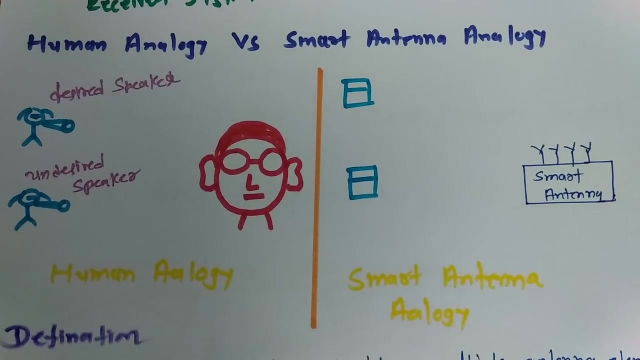 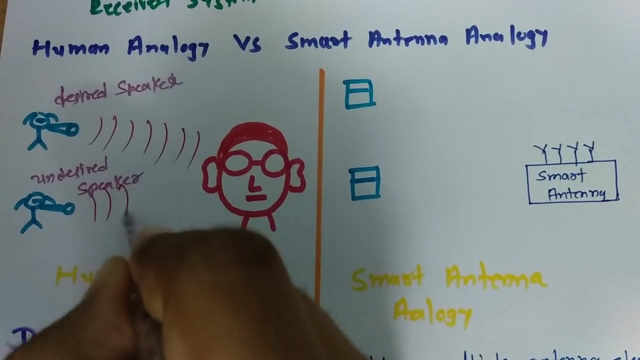 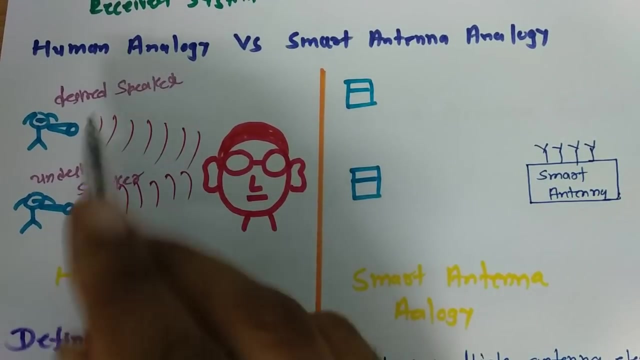 And out of this multiple speaker, this is desired speaker And this is undesired speaker. Now, what happens here? when these speakers are sending signal to this human, then what happens is this human cannot justify which signal that is coming from desired direction and which signal that is coming from undesired direction. 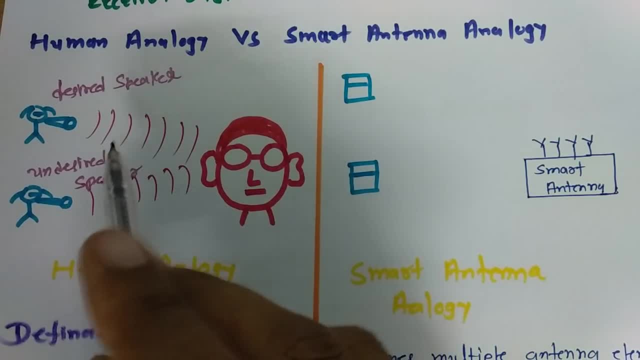 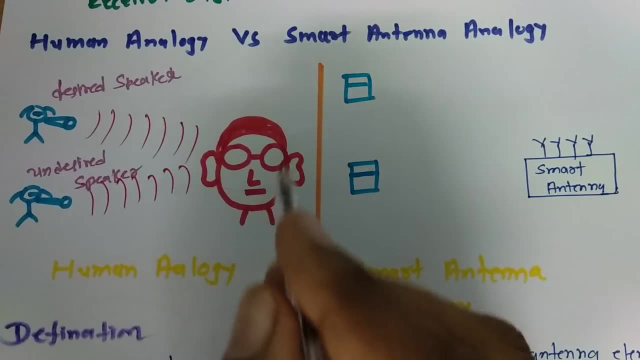 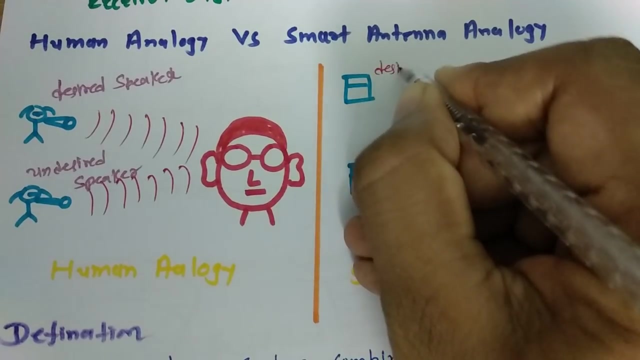 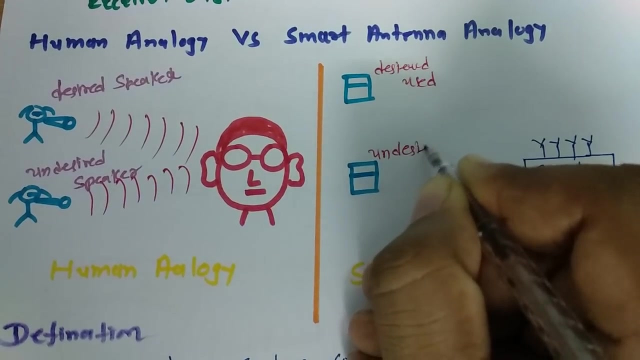 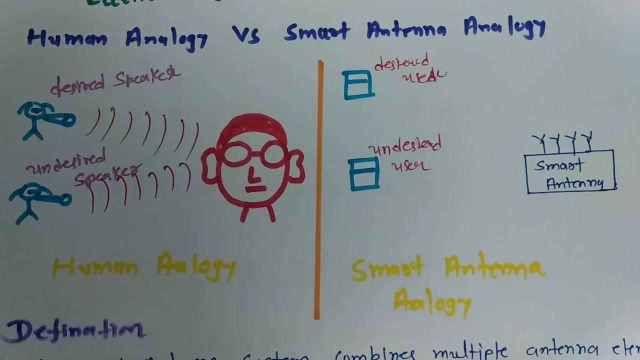 So it is very difficult for this human to identify which signal is coming from desired direction, So that signal cannot be extracted. But when we talk about smart antenna technology, and if we have desired user, an undesired user, so in that case what happens is: 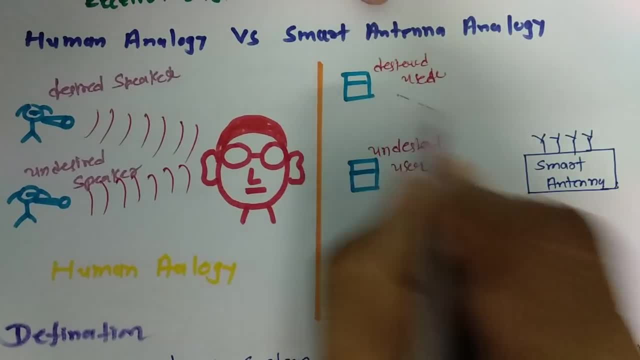 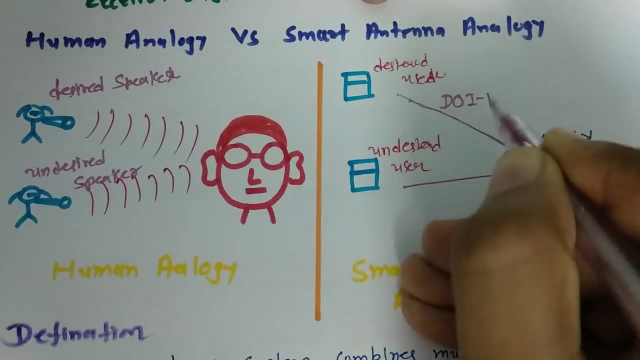 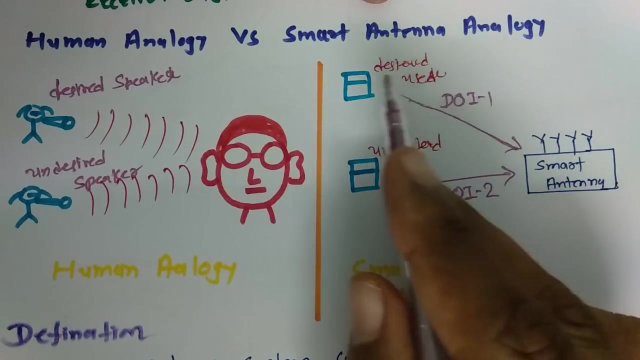 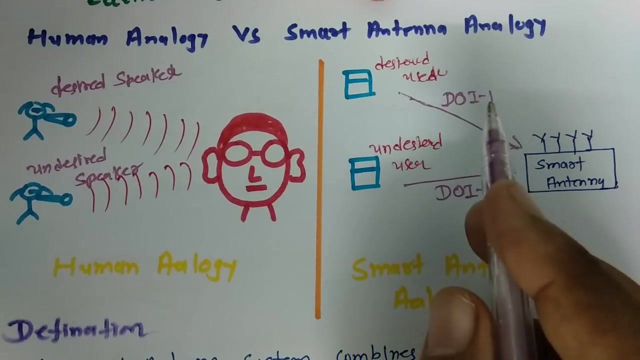 when there are multiple signal that is coming as a direction of arrival. this is direction of arrival 1, and this is direction of arrival 2.. So, once this direction of arrival that is coming from desired as well as undesired user, this smart antenna will justify what is that desired direction of arrival. 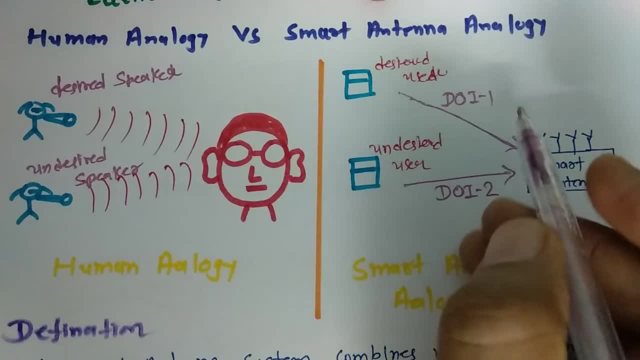 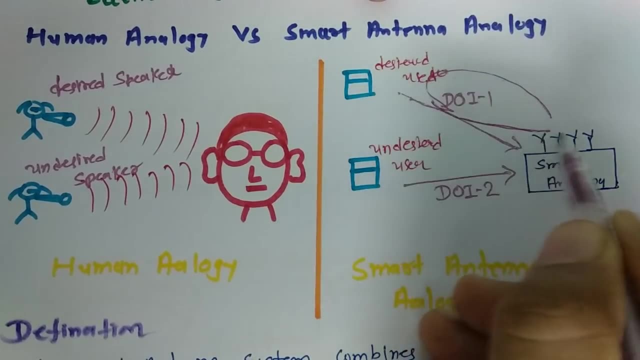 And once it justifies desired direction of arrival, it will be focusing its beam in desired direction. So now one can see its beam that is getting focused in that direction. So now one can see this is what direction of arrival and based on that it focuses its beam in desired direction. 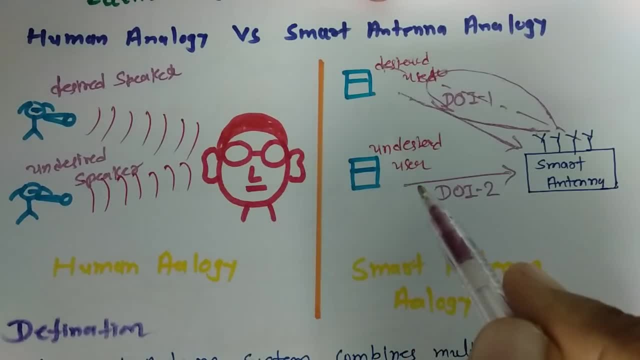 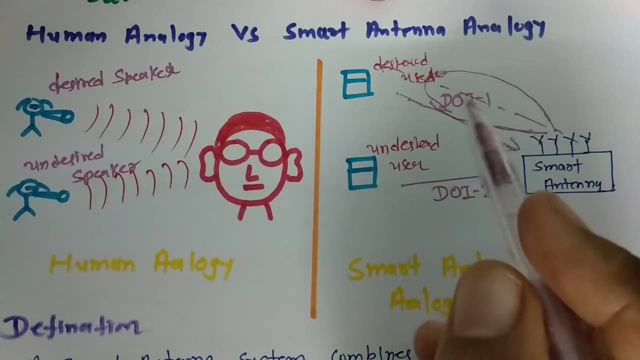 So undesired user that is getting animated from the radiation. So ultimately now this smart antenna technology that does what: It sends signal in desired direction with respect to undesired direction, So it minimizes interference from undesired user, So which one can observe over here. 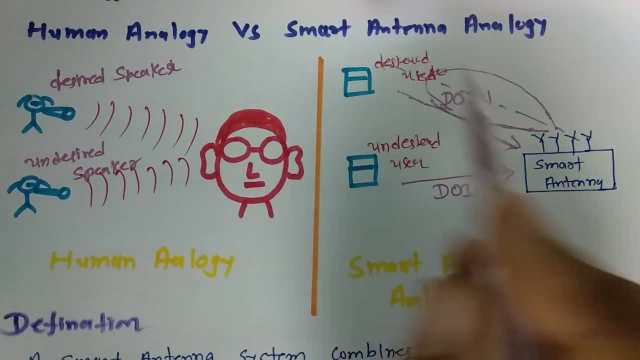 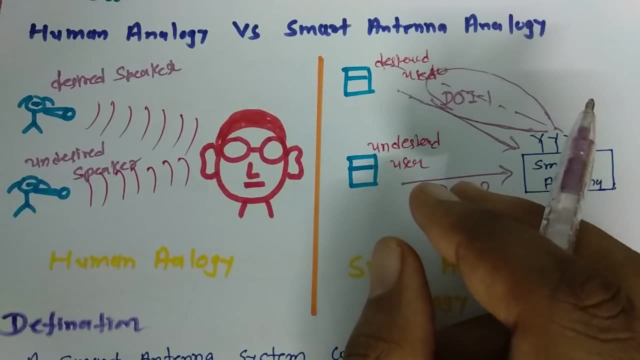 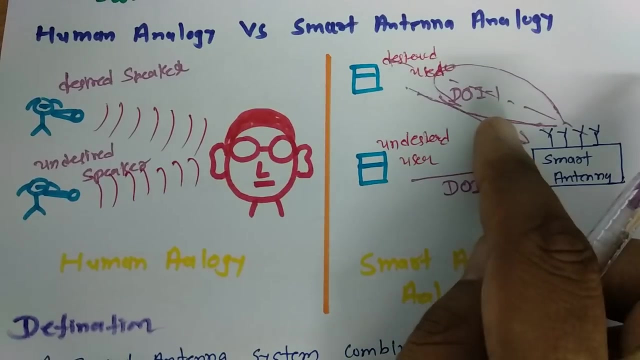 That's why it is smart. What is smart in this antenna Smart thing is it only radiates in desired direction, And that happens because of DSP. processors are justifying the value of magnitude which is there with phase shifter, And that is how it identifies what is that desired direction in which it needs to radiate about. 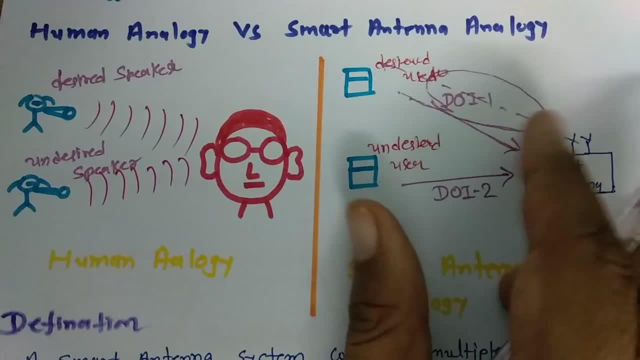 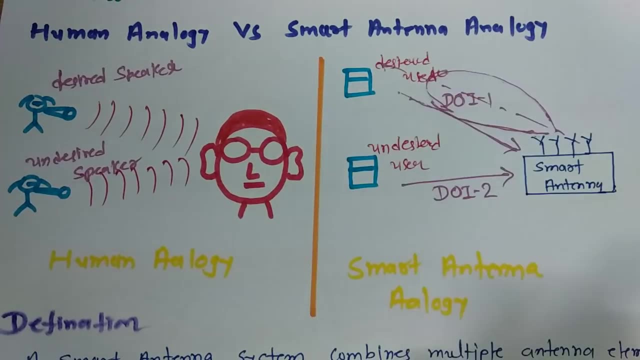 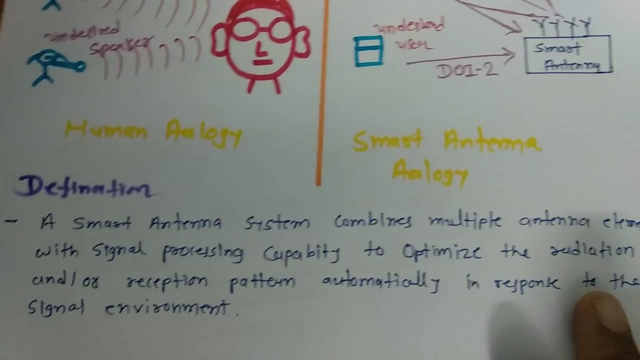 And then it starts to radiate in desired direction, So it will be having maximum gain in desired direction. So this is how smart antenna functions And this is what the basic analogy which is there with human and smart antenna. Now I have written one basic definition here, which is therefore smart antenna. 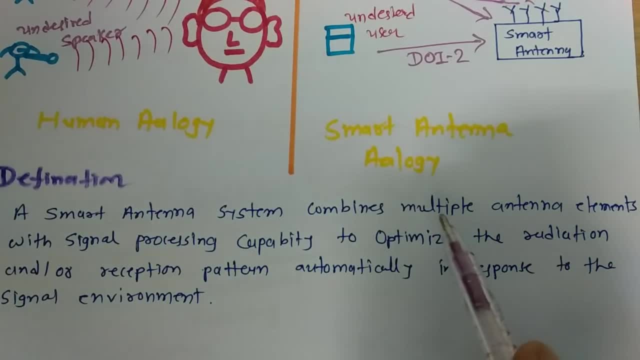 Smart antenna systems combines multiple element of antenna with a signal processing capability, And that is to optimize the radiation and our reception pattern automatically in response to the signal environment. Now, here, everything is happening automatically. There is nothing, which is what we are controlling manually. 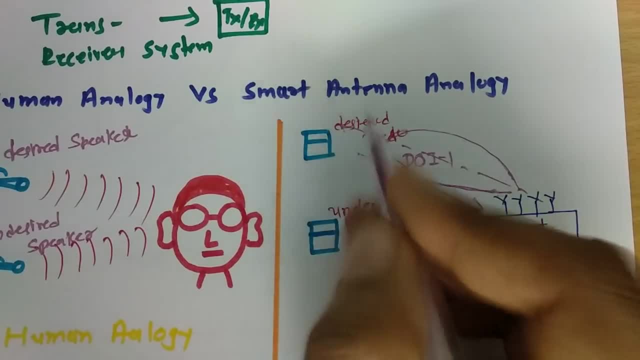 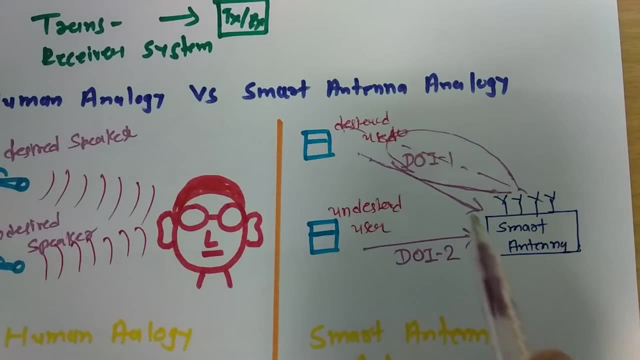 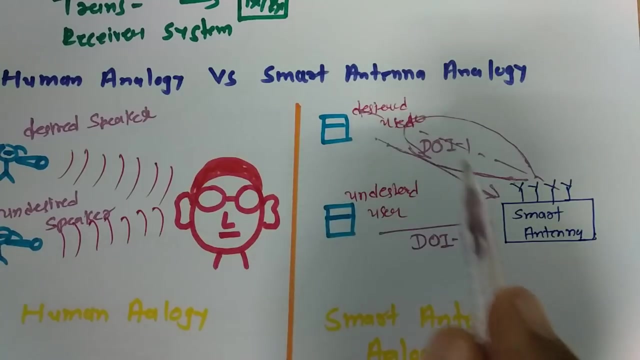 Like see, for example, here we have desired user and it is what there, in this direction, So based on direction of arrival, smart antenna justifies. this is what the direction in which it needs to radiate about, And once it justifies that desired direction of arrival, it focus its beam in that direction. 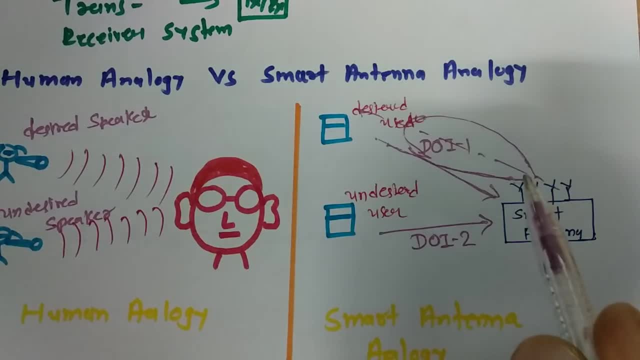 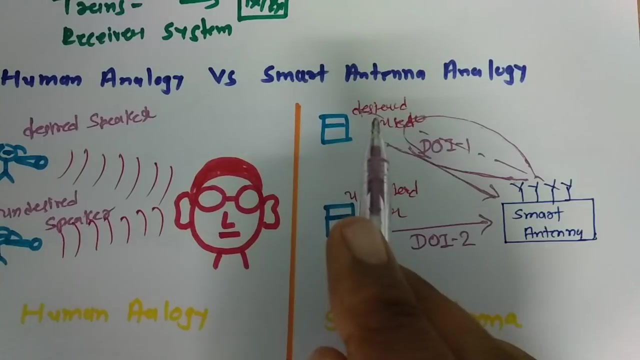 And that is what it is doing by antenna, By antenna phased array plus DSP processor, where DSP processor does signal processing to calibrate value of magnitude of phase shifter And based on that, it focus its beam in desired direction. So that is how this smart antenna technology is functioning. 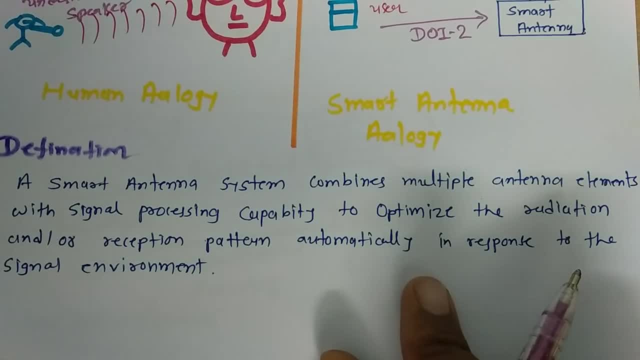 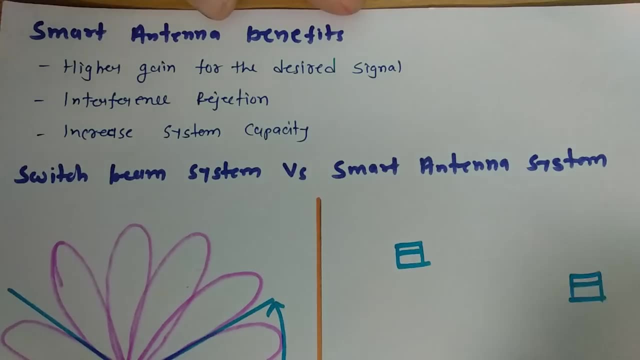 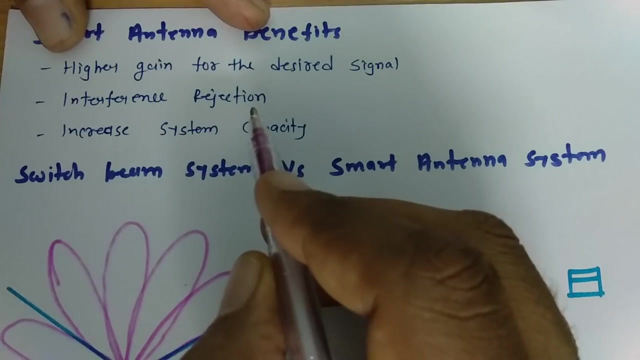 And this is what the basic definition which is there with smart antenna. Now let us move on to few more things. What are the benefits? So, as I have discussed few benefits, It has higher gain in desired direction. Interference rejection is there. 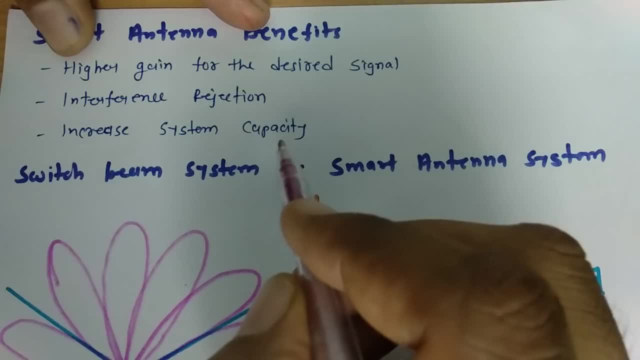 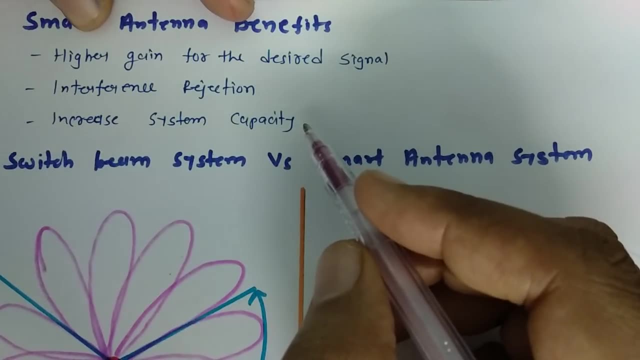 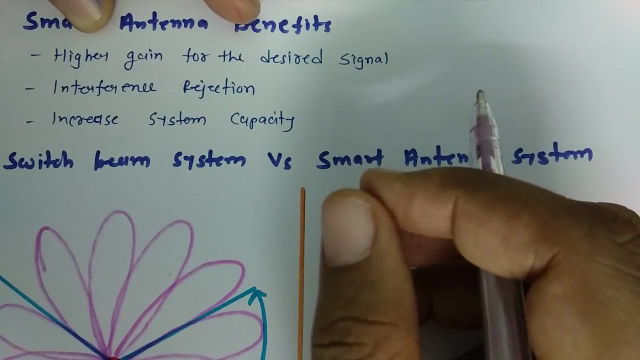 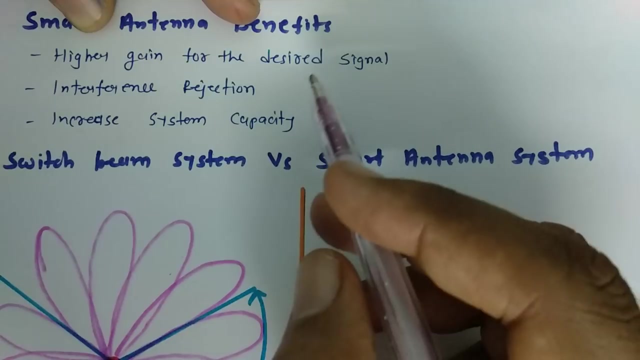 Increased system capacity, How it increased system capacity. It can increase system capacity by focusing in desired direction. So sometimes what happens is in cellular system, more users that is happening in some particular region. So if our antenna is not smart, In that case what happens is at tower side. it cannot justify where it should give maximum magnitude. 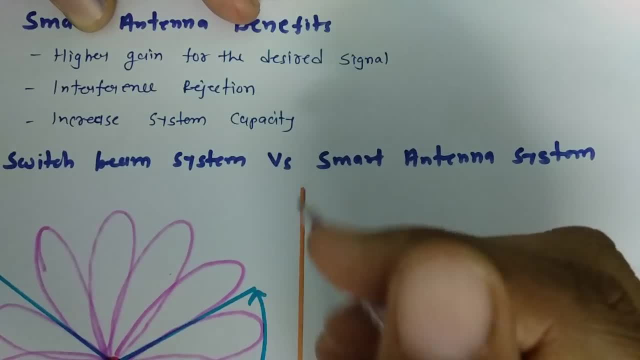 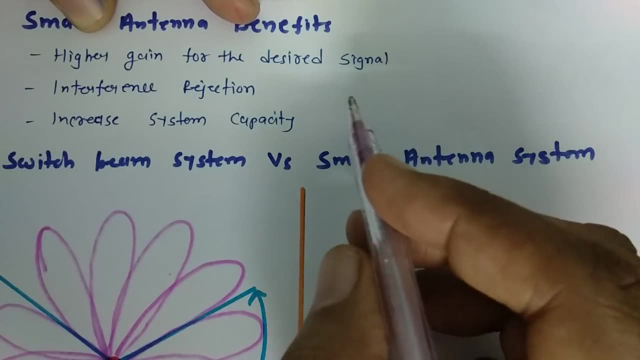 And based on that, if its magnitude is uniformly distributed, in that case capacity of system that is fixed. But by using smart antenna where more users are there, In that case we can focus more in that region where number of users are more. So that is how it increases capacity of system. 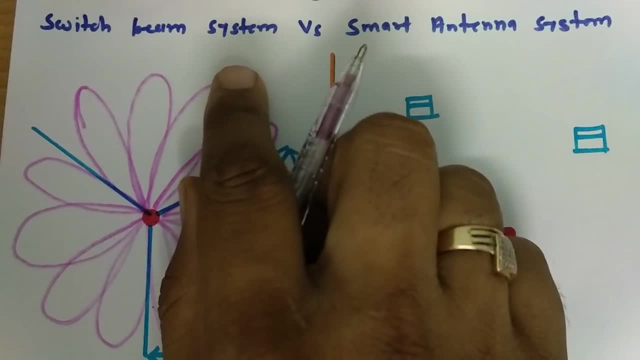 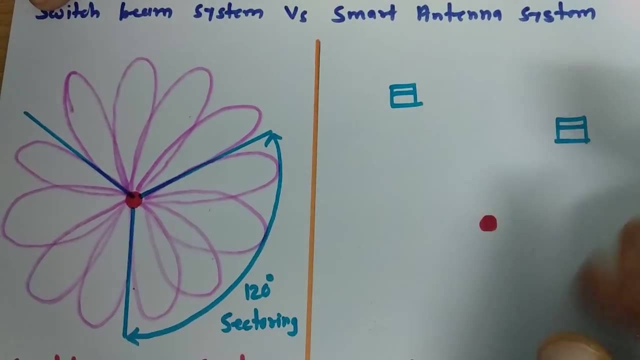 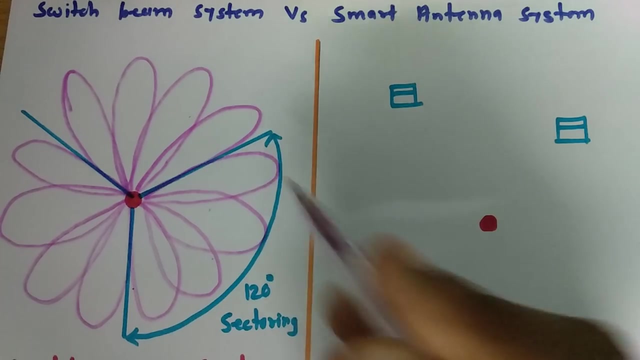 So to understand that, let us have two system. One is switch beam system and second is smart antenna system. This switch beam system that is already there in cellular system, Where what we do is we provide cell sectoring. Here I have shown 120 degree cell sectoring. 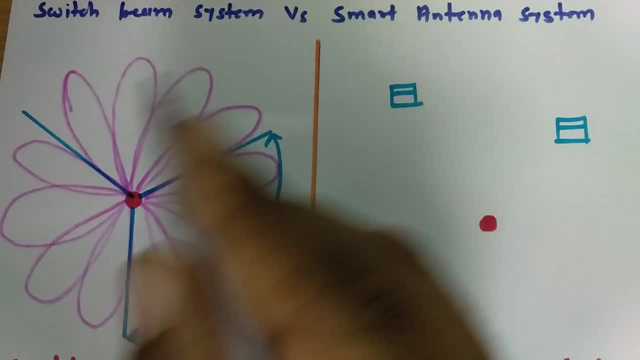 So in three direction it is been divided with respect to 120 degree. So this is what? 120 degree, This is one another 120 degree And this is third one, another 120 degree. So that is how cell sectoring is there. 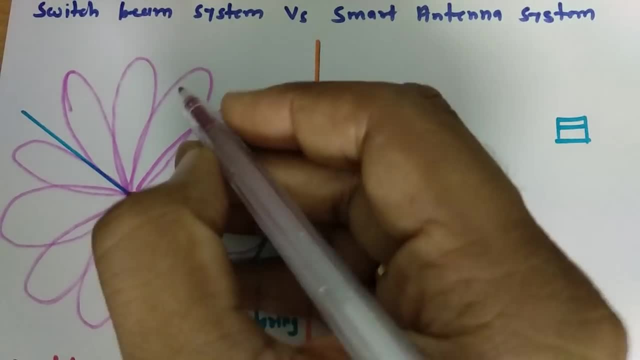 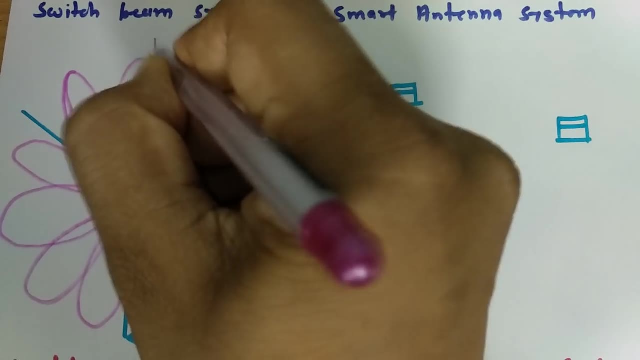 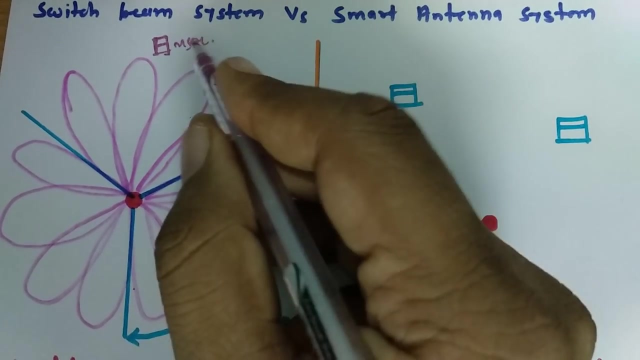 In switch beam system there are fixed beam, So these are fixed beams in which this system is radiating. Now what happens when user comes over here? Let us say, one user is entered over here. So when this user entered over here, What happens is it will be focusing on this user, based on fixed beam. 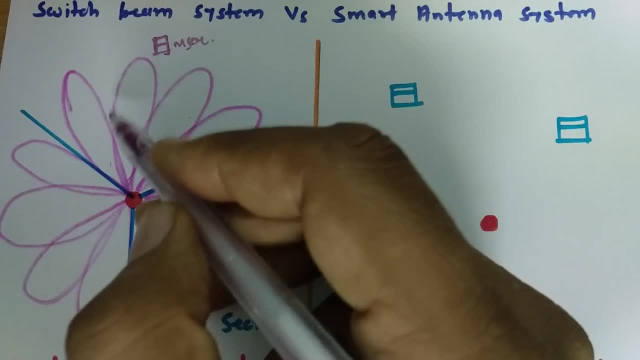 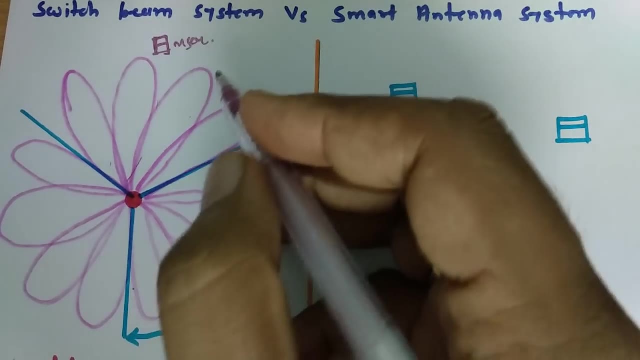 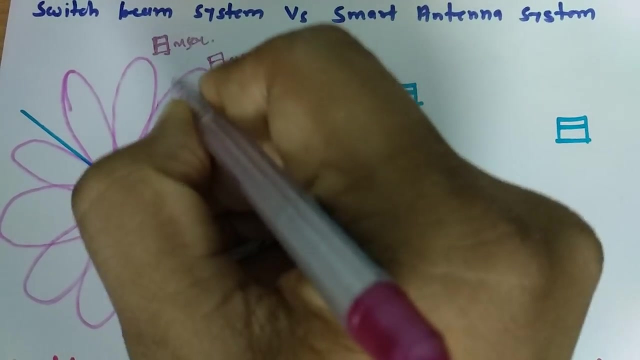 So if this beam That is having amplitude of gain in the vicinity of this user, In that case this user will be receiving signal. And if multiple users are entering, In that case even beam pattern will not change. Like see, I am showing over here. 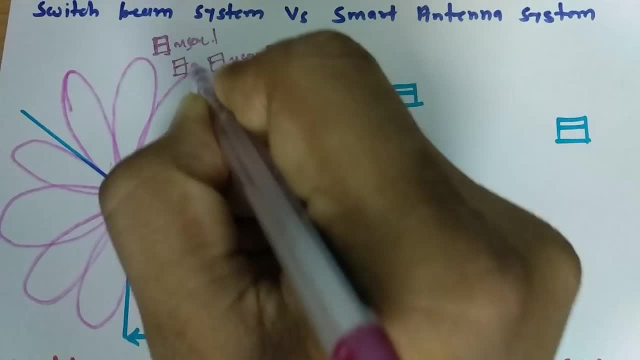 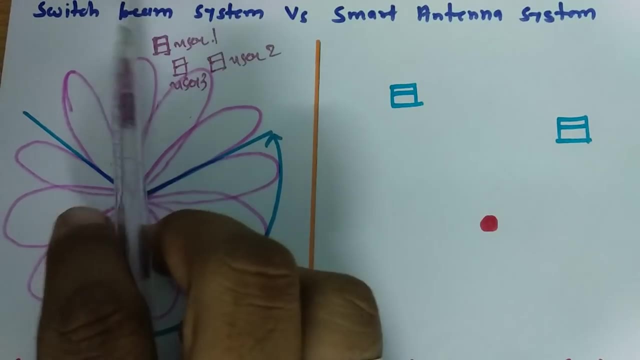 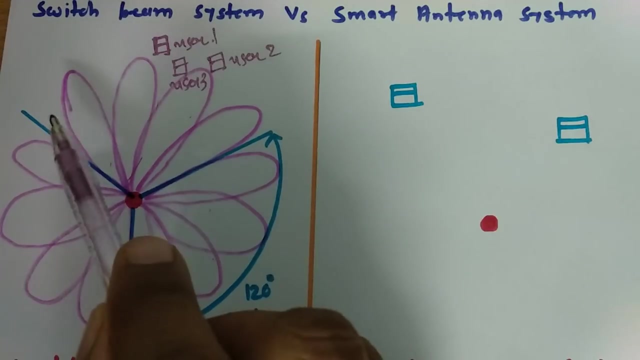 There are multiple user: This is user one, This is user two And this is user three. So multiple users are entering over here. Still, beam is in fixed direction. So this beam, that will not change, So it will be having fixed amount of range. 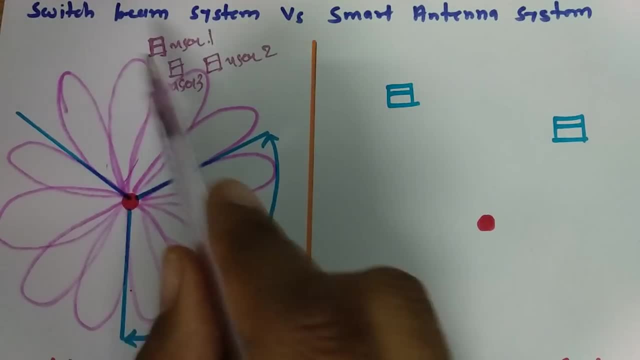 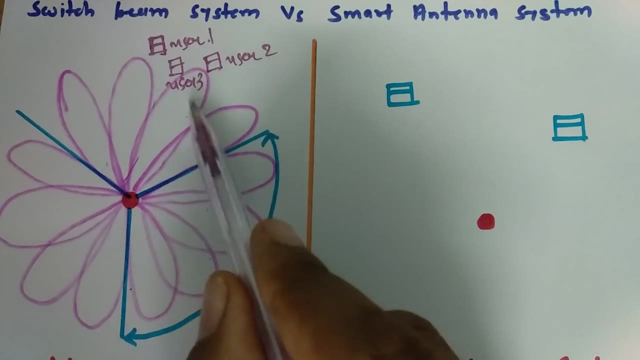 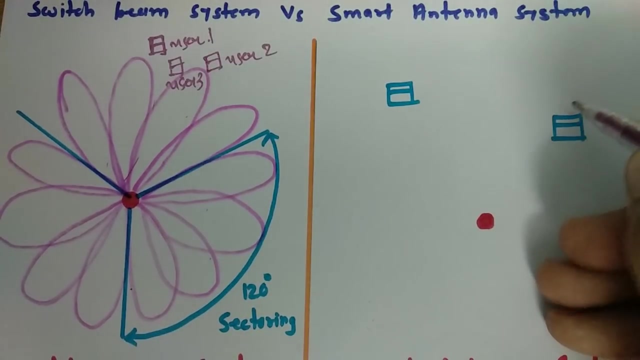 As well as fixed capacity of system For this switch beam system. So, for example, if users are entered here, In that case this beams are getting activated And that will be focusing those users. But what happens in smart antenna First if I say user entered over here? 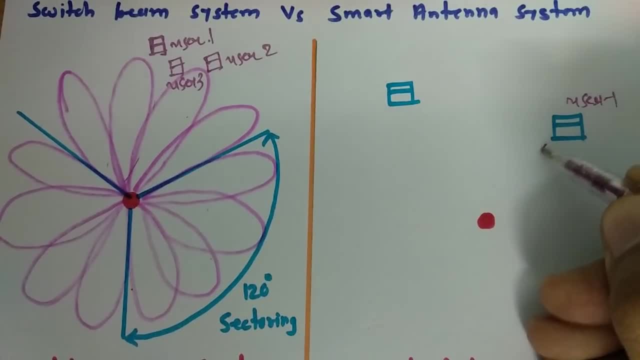 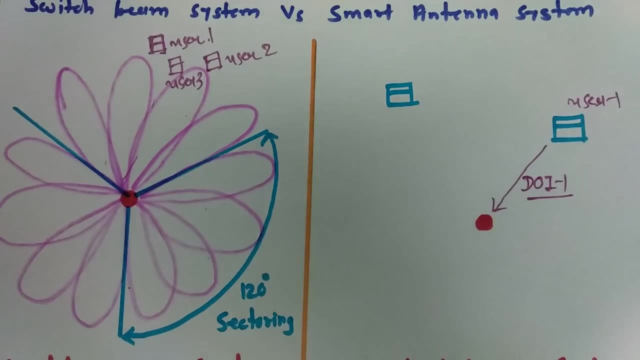 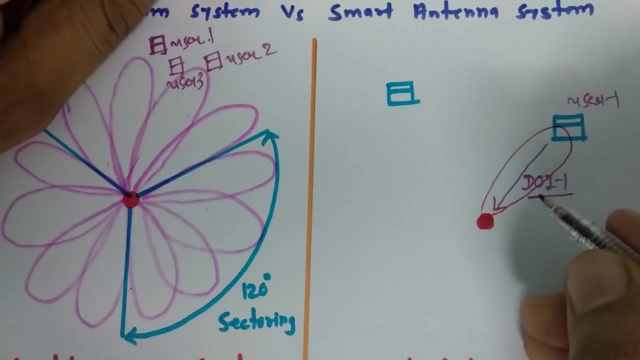 Let us say user one is entering over here And based on that There will be a calculation of direction of arrival One. And once it calculates direction of arrival It will focus its beam in this direction, So it is not radiating in all direction. 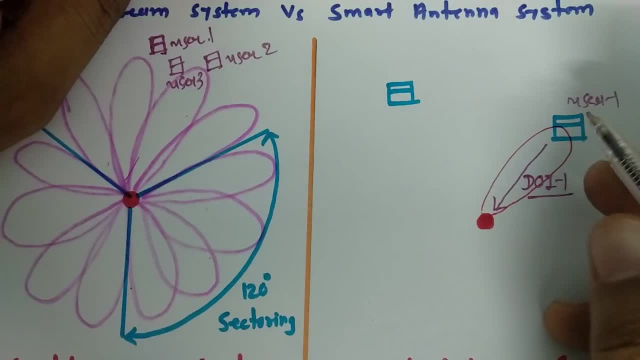 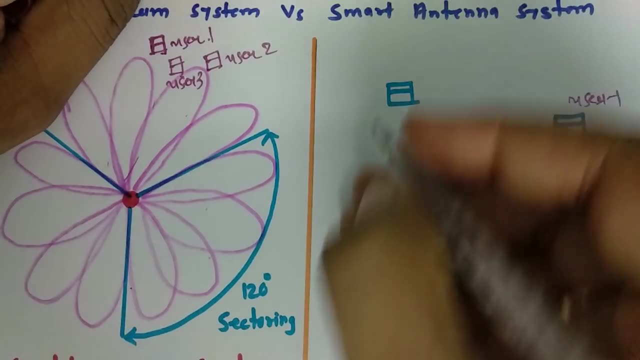 It radiates based on user Which is there in system. So if user is there in this direction, In that case its beam is getting focused in that direction. Now if second user is entering, Let us say user two is entering Here. 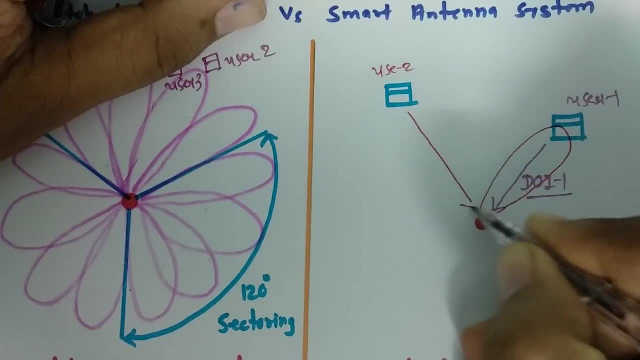 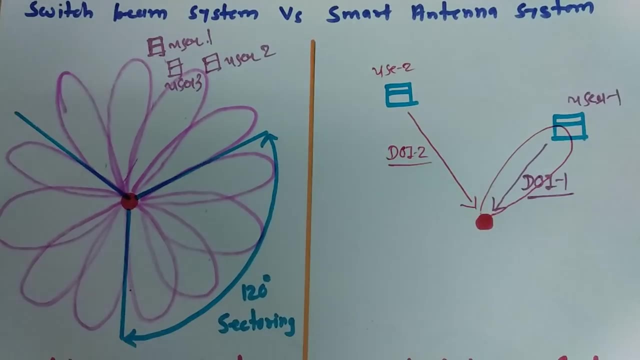 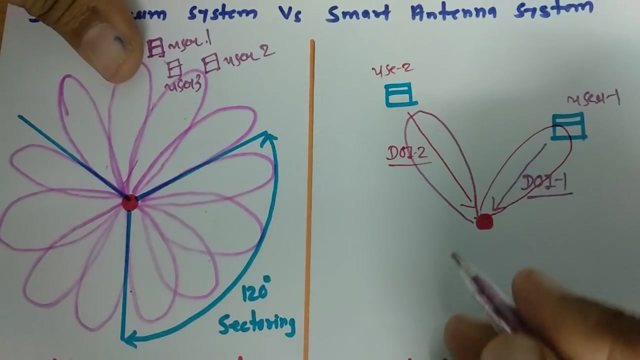 So in that case That will be having another direction of arrival. So direction of arrival two: So that is what coming from this direction, So this smart antenna Which is over here, That will be radiating beam In this direction. So, ultimately, 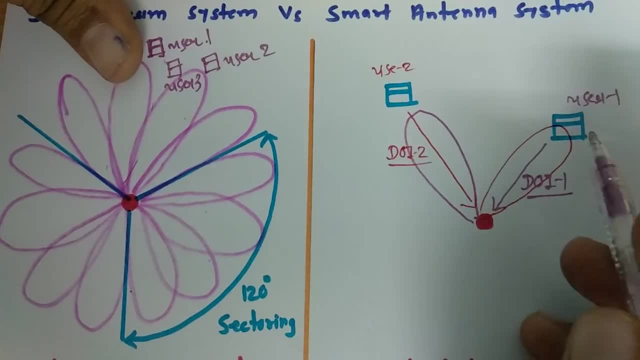 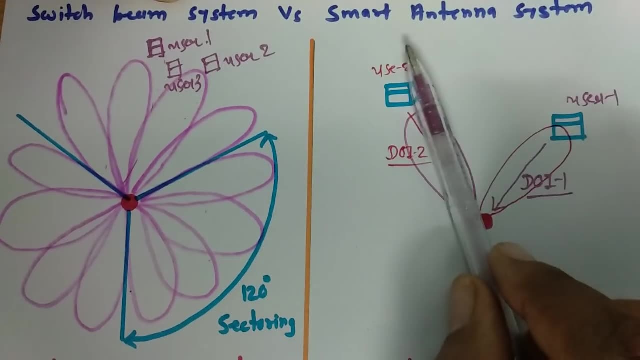 This beam formation that is happening in the desired direction only It does not radiates in all direction. Now, here, For example, If number of users are more in this direction, In that case Beam intensity that will be more in this direction. 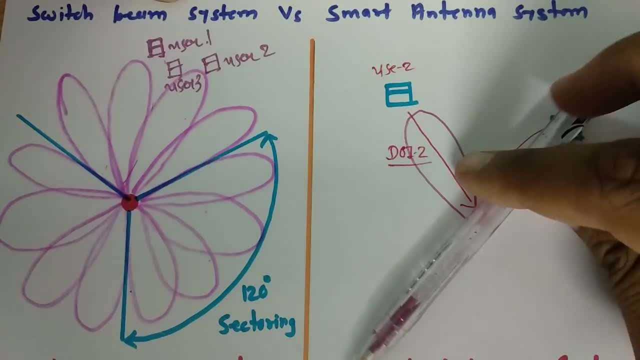 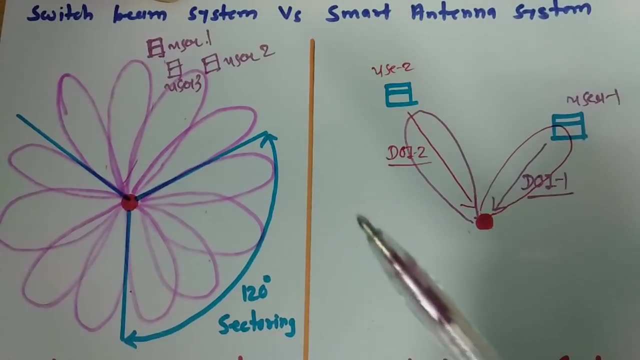 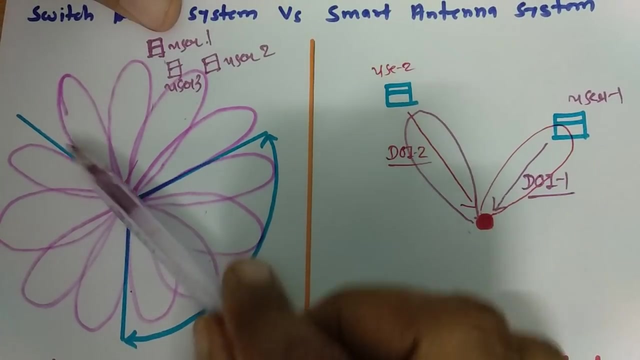 If less users are there in this direction, Then beam formation will be less With its intensity in this direction. So ultimately It increases capacity of system Like see, for example, If I say For this switch beam system If it can focus for 120 users in this direction. 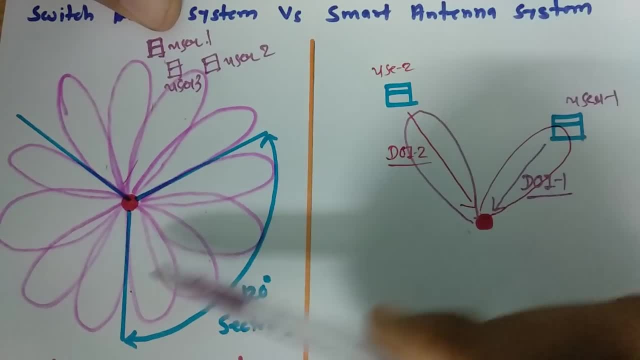 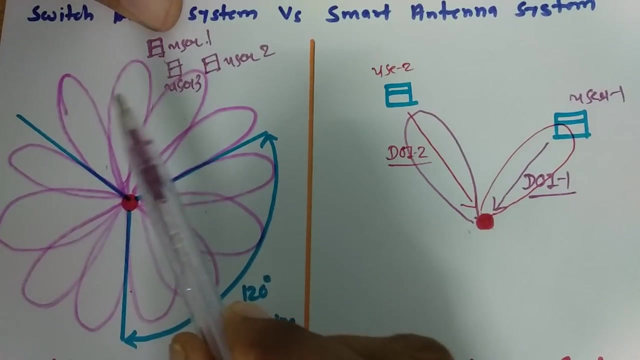 120 users in this direction And 120 users in this direction. So overall total system capacity is 360.. But let us assume one case Where 200 users that have entered in this region. So what happens? It cannot give service to 200 user at a same time. 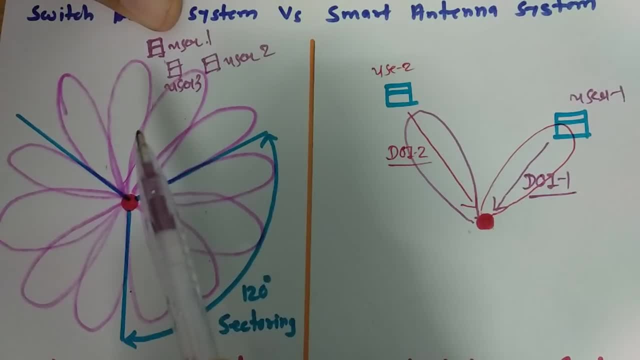 In this region. The reason is this region is having capacity of 120 user, So It can provide service to 120 user only And rest user will have to wait To get Free time of that system Once it get free. 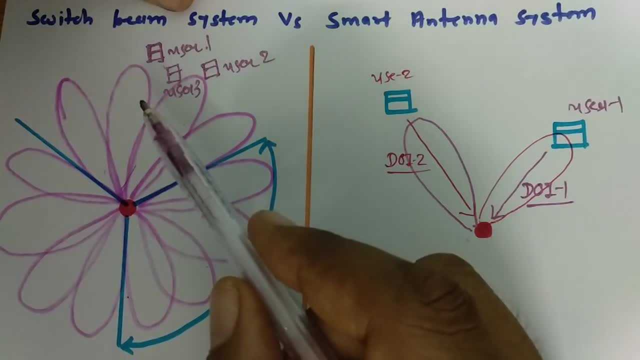 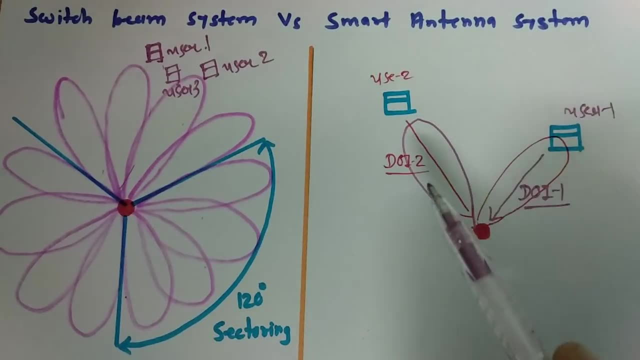 Once it get free, It will be providing service to those users. But in case of smart antenna, As in overall direction, Capacity of system is 300 user. So even if 300 users Those are focused in this direction, This system can provide service to all those users. 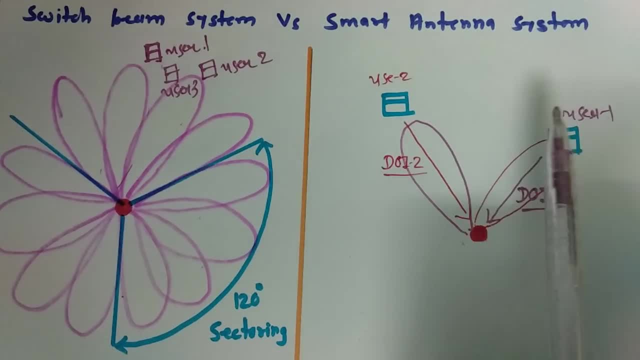 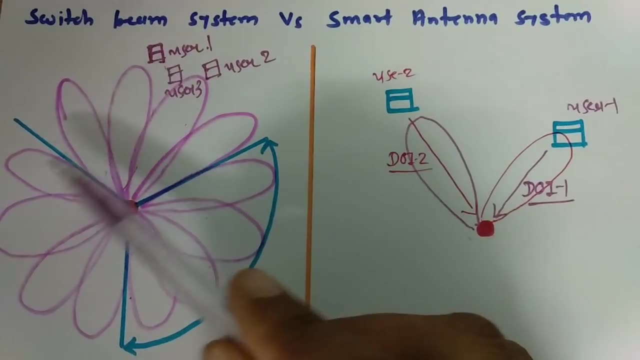 The reason is it is not depending Fix in all direction. Where in switch beam system It is not giving service to all those users. Where in switch beam system It is fixed for certain direction And it can give fixed service in certain direction. 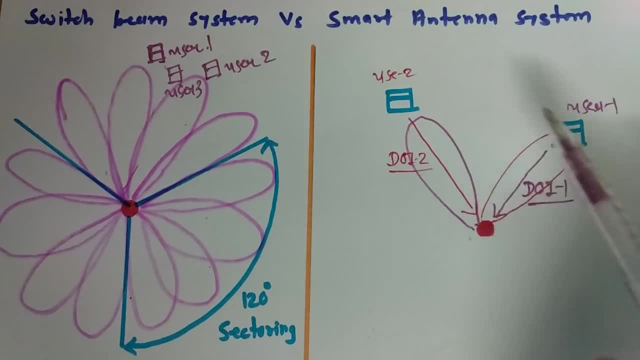 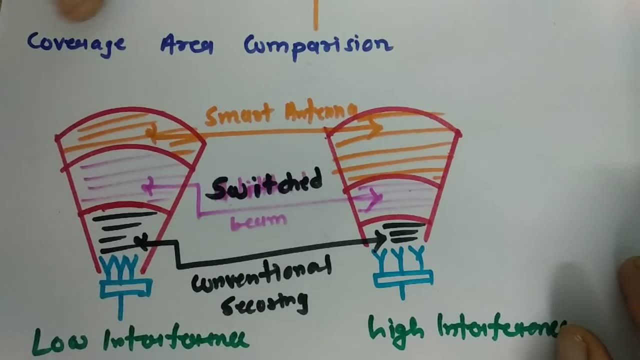 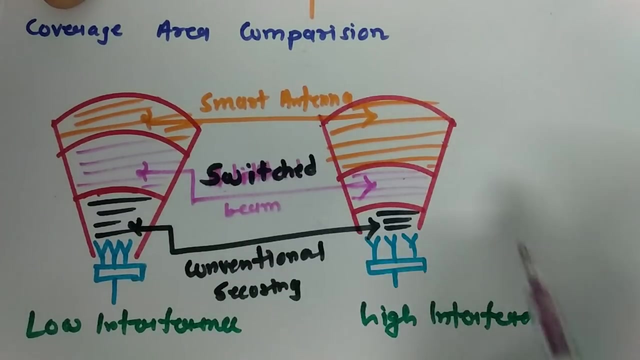 So here overall systems capacity That is getting increased by smart antenna system. So I have given some comparison here, Coverage area comparison For low interference as well as for high interference. Now one can see For low interference as well as for high interference. 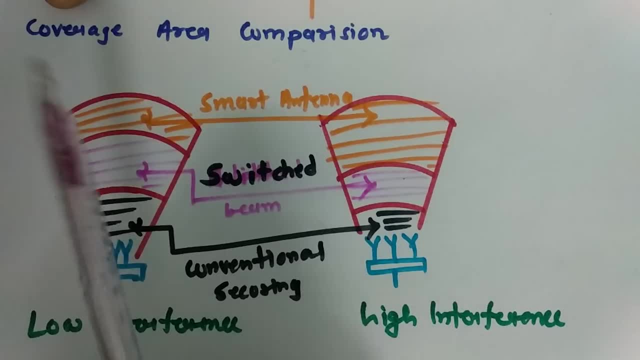 This coverage area That is fast. That is far higher for smart antenna. In both of the cases, Like see for low interference Antenna coverage area That is having larger distance And in that case even That is having larger distance. 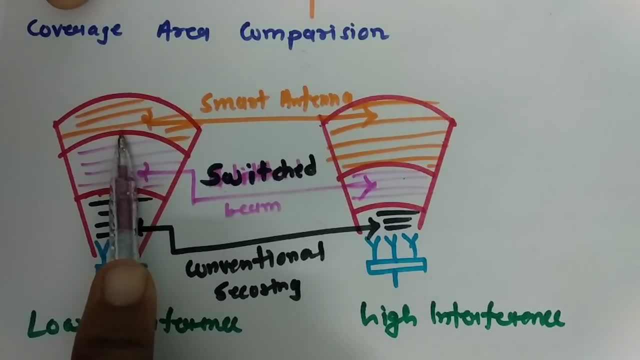 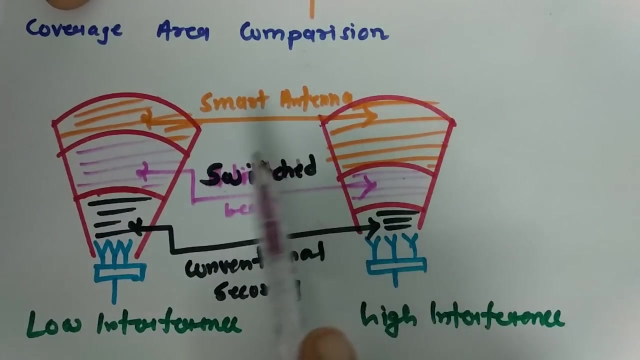 For low interference switch beam Functions effectively, But it cannot functions Effectively higher than smart antennas. Even in low interference region Smart antenna functions better than switch beam system And for high interference, Capacity of functioning For switch beam system decreases. 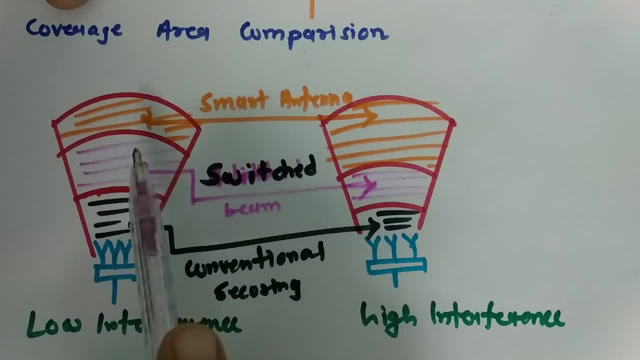 That one can see here. Switch beam system functions well In low interference, While in high interference It is having lower Response For that system, While smart antenna functions pretty well In both of the cases, Where interference is low As well as interference is high. 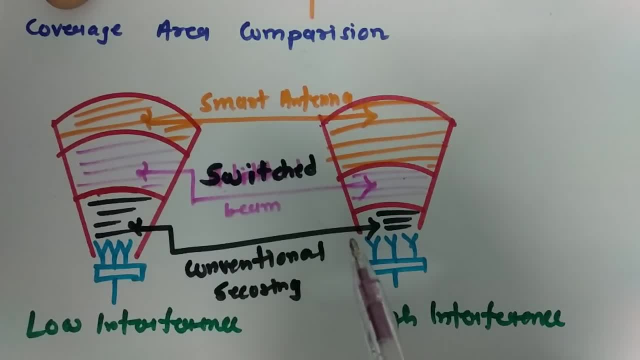 And coverage area For conventional sectoring That is far low. So switch beam system That is having better response In low interference, But at high interference Its range is getting decrease, While smart antenna Can functions very well In low interference environment. 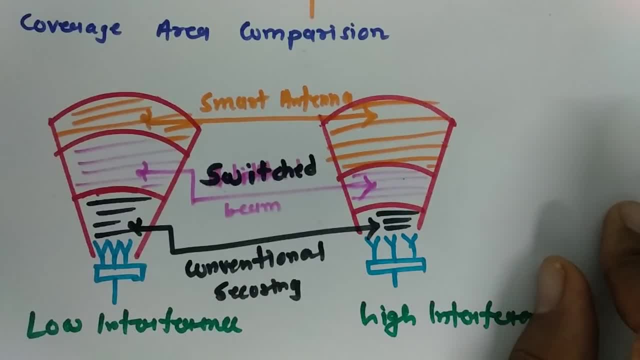 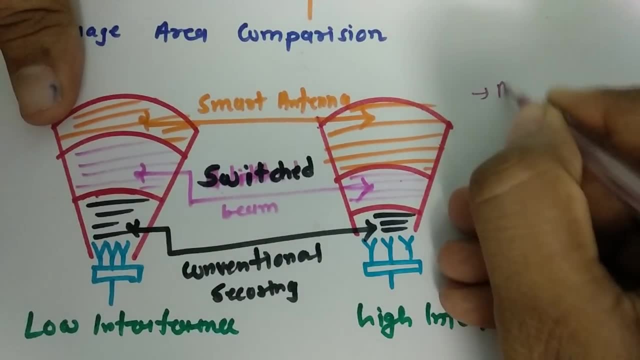 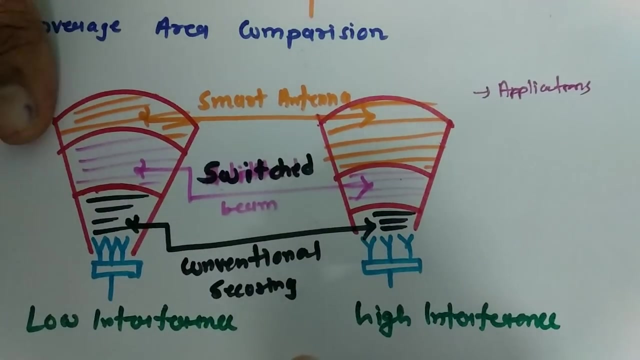 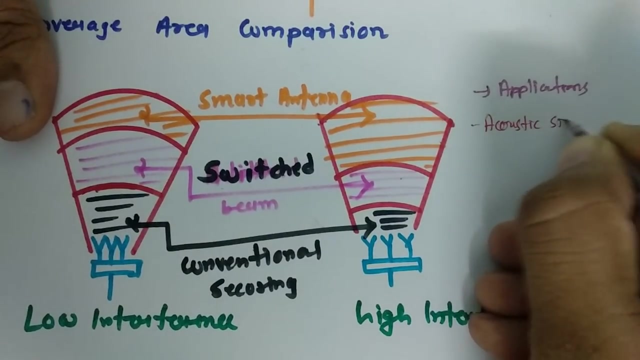 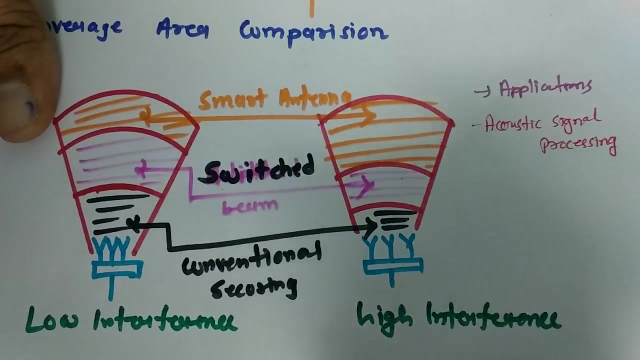 As well as in high interference environment. So this is how Smart antenna technology functions. Now I will be explaining you Few applications Which is there With Smart antenna. So it could be used In acoustic signal processing. It could be used in tracking of radar. 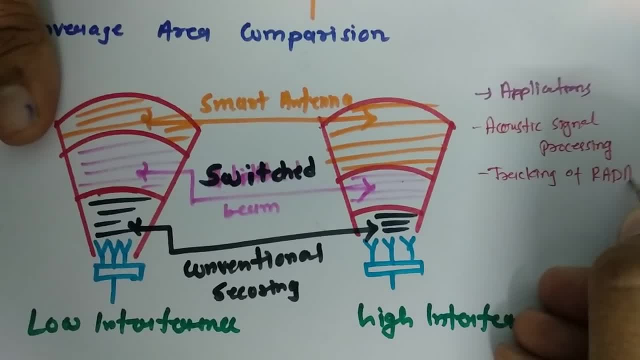 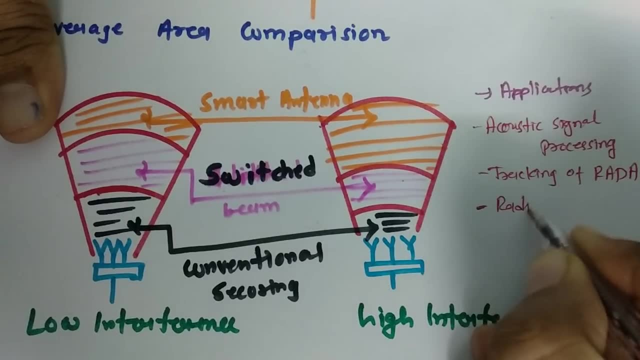 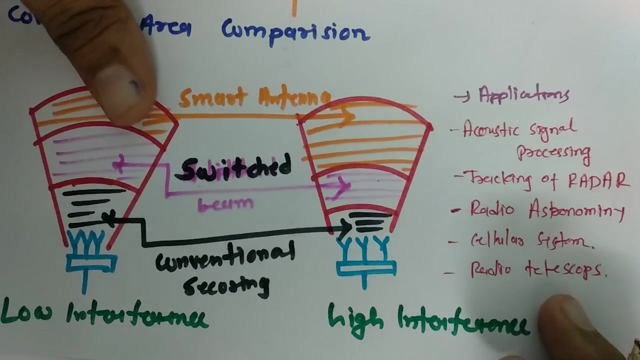 It is been used In radioastronomy, In cellular system Even we can use it, And in radio telescope We can use Smart antenna System. So these are very much important applications Which is there with smart antenna. Thank you so much for watching this video. 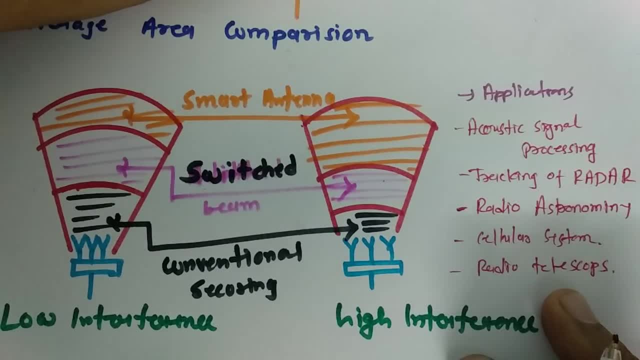 You can find All those material Which I am teaching here In my website. Link of website is attached With the description of this video. So just see description of this video, Where you will be finding website Where you can download all materials.